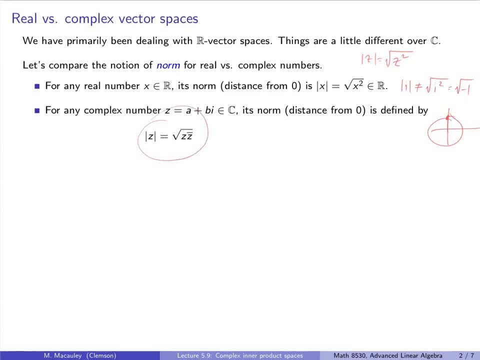 Well, here's the right way to do it. It's the square root of z times z bar, That is the square root of a plus bi times a minus bi. And that's just the square root of a squared plus b squared. So remember, in the complex plane, if z is a plus bi, then it's a complex conjugate. 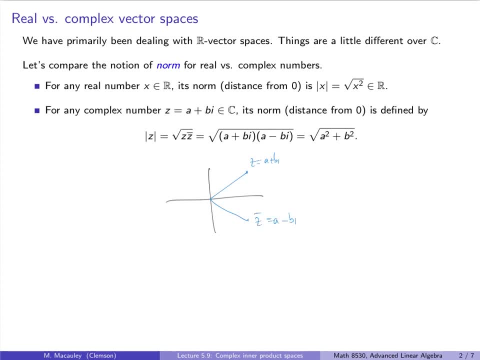 z bar is a minus bi And angles add and lengths multiply. So if you multiply z times z bar, if this is theta, then this is negative theta, So the angles add and you will end up getting something on the, on the real line. 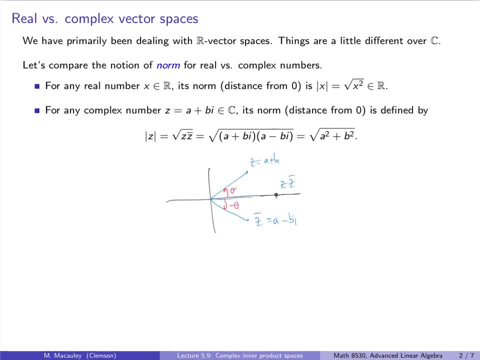 So this will be z times z bar, And its magnitude or its norm is going to be the square of the norm of z z bar, And the angle is going to be 0 degrees and hence real. We just compared r to c. 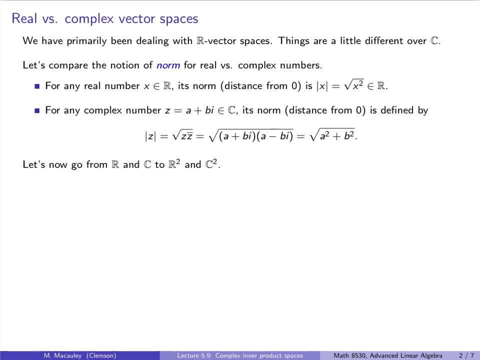 Let's now compare r2 to c2.. For any vector x in r2, its norm, or just the distance from z or the 0 vector we'll use these double bars, is the square root of the inner product of x with itself. 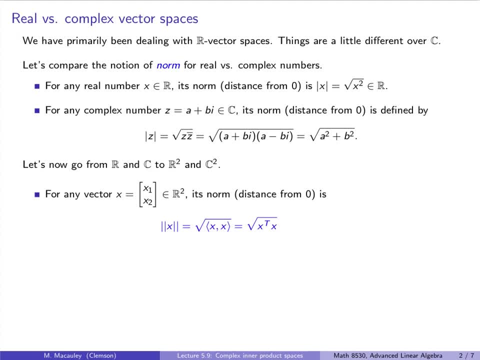 or the square root of x. transpose x or the square root of x1 squared plus x2 squared. In contrast, for any vector z in c2, with entries z1 and z2, let's say z1 is a plus bi. 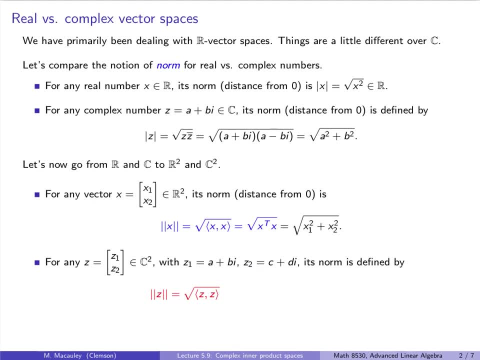 and z2 is c plus di. its norm is also defined- it's written the same way- with these double bars- as the square root of the inner product of z with itself. However, this inner product, as we'll see, has to be defined a little bit differently. 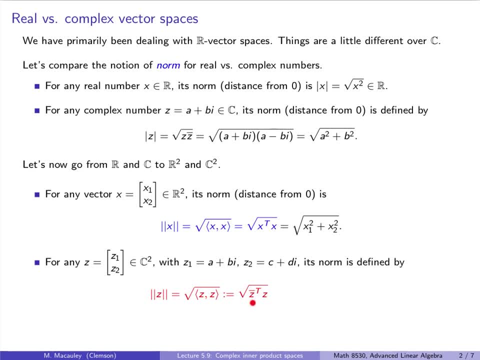 So this is the square root of z bar transpose, that's the conjugate of z transpose times z, And that's the square root of the norm of z1 squared plus the norm of z2 squared. To understand this, I think it's best to compute two examples. 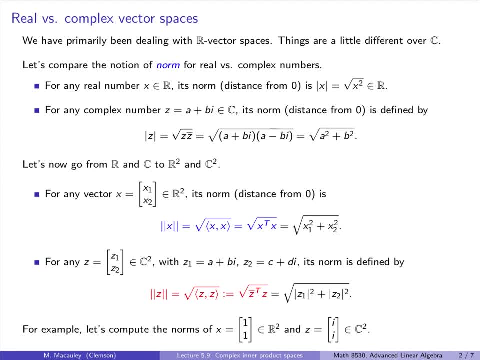 We'll start with the norm of the vector 1, 1 in r2, let's do that right now. So the norm of x here is the square root of the inner product of 1, 1 with 1, 1.. 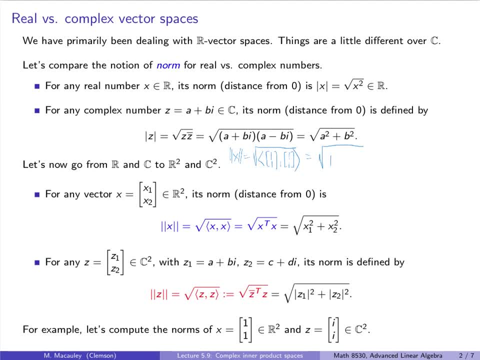 We know how that goes. that's square root of 1 squared squared plus 1 squared, which is the square root of 2.. In contrast, the norm of this vector z, which is ii- let me do that in red. 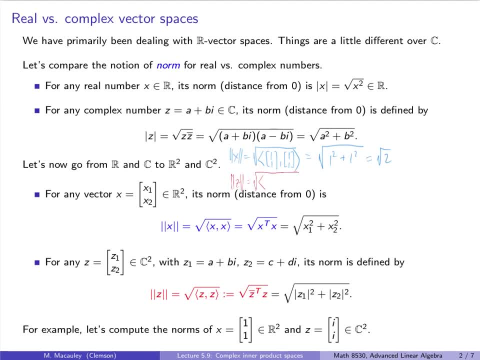 That is also the square root of the inner product of this vector with itself. So I'll write ii with ii. But notice what happens if we just try to do the standard dot product. So that would be i squared plus i squared and that's the square root of negative 2.. 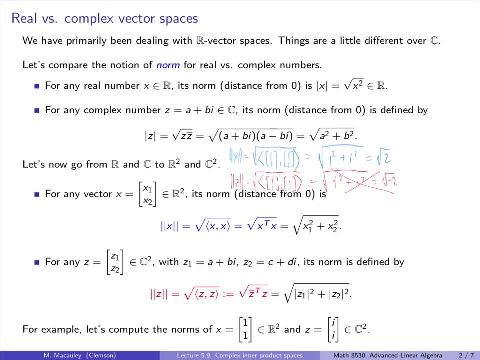 And that's not real. So that is not what we want. Instead, what we want is take the conjugate transpose, So in other words, the square root of. let me actually write that as i. Well, let me remind you that the complex conjugate of i. 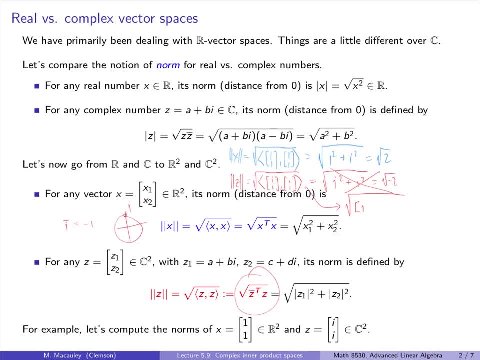 is negative i. So in the complex plane, if this is i, the complex conjugate is negative i. So that's negative i, negative i the dot product of that or the inner product with ii, And this is 1 plus 1 equals root 2, as it should be. 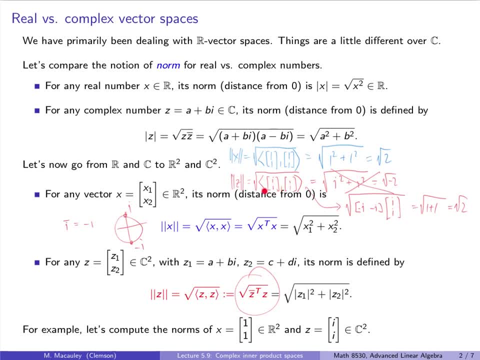 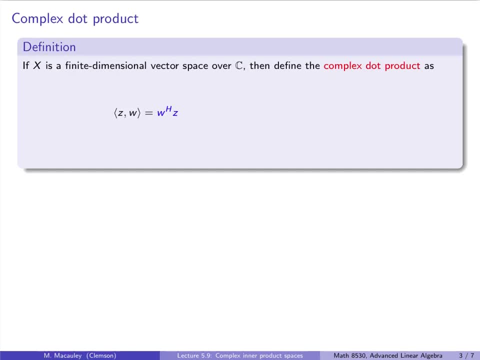 So now I've here I'm using not just any abstract inner product, I'm using the standard dot product here, And that leads to a definition. If x is a finite dimensional vector space over the complex numbers, then we'll define the complex dot product as follows. 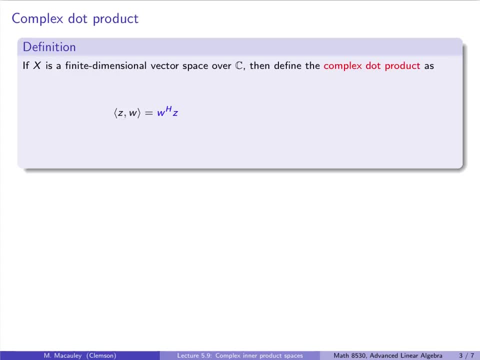 So the dot product of z with w. we will write this as whz instead of w. transpose z: wh is 0.. Just short for the transpose of the complex conjugate of w. And so you literally take the transpose of w and the complex conjugate of each entry. 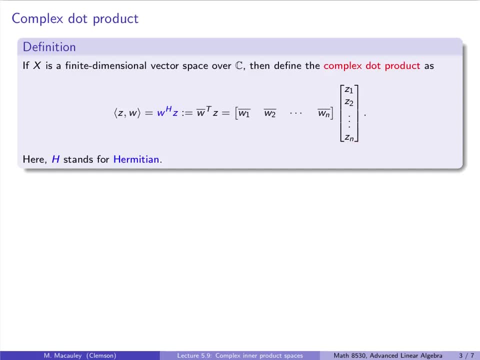 and multiply that by the vector z- Here h stands for Hermitian. Using the definition of the complex dot product, we naturally get a definition of the norm of a vector z. in Cn It's easier to define It as the norm squared. 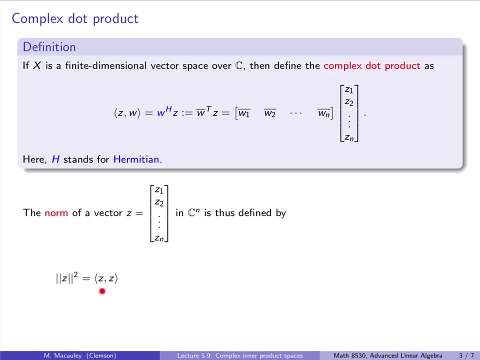 So the norm squared of z is the inner product of z with itself, which is z conjugate transpose times z, which is the product of the row vector z bar times z, which is the sum of the norms of the individual entries in z, z1. 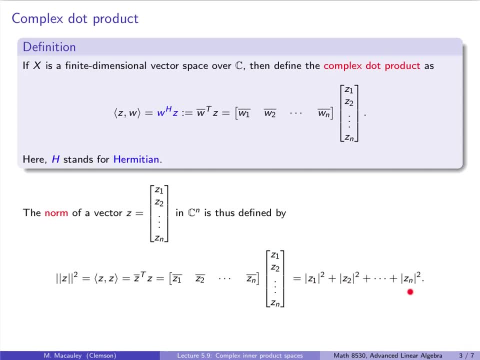 up to zn, So z1 squared plus z2 squared up to zn squared. Notice how: if our vector z has only real valued entries, then this definition of norm agrees with the definition of norm over a real vector space. So we're not changing the definition. 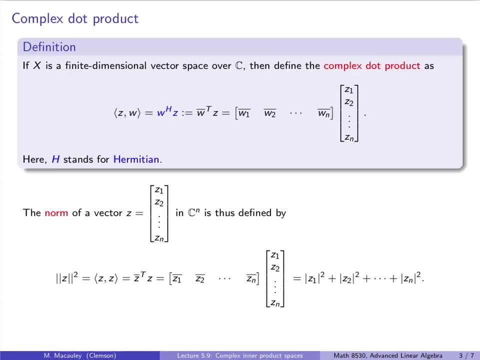 We're just extending the definition when we are in a vector space and our entries don't have to be real but can also be complex. Next, just like how we abstracted the dot product to a real inner product, we can abstract the complex dot product. 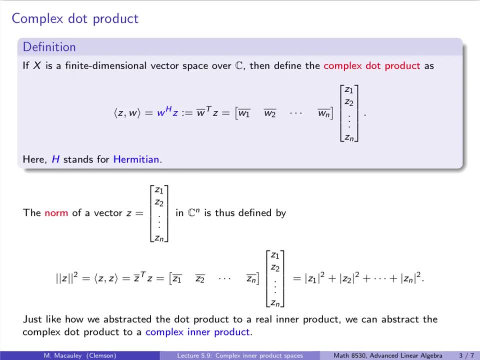 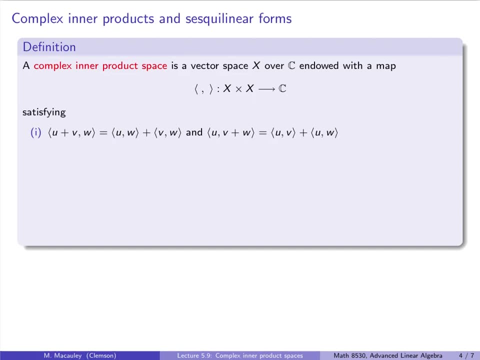 up here to a complex inner product. Here's the formal definition: A complex inner product space is a vector space over C endowed with a map. We'll use brackets for this, From x, cross x to the complex numbers, satisfying the following: First of all, it is additive, just like for real inner products. 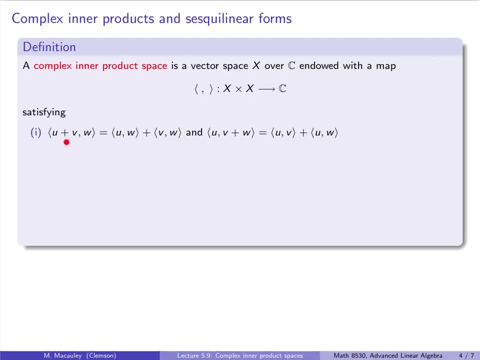 In other words, the inner product of u plus v with w is the inner product of u and w plus the inner product of v and w, And the same thing in the other coordinate: The inner product of u with v plus w is the inner. 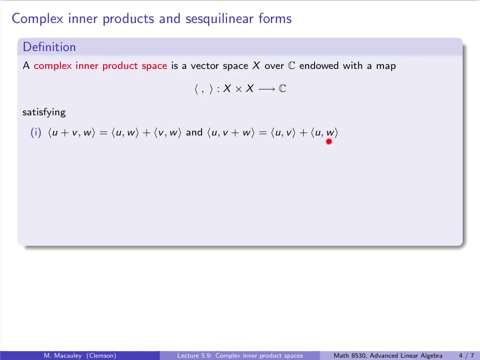 product of u with v plus the inner product of u and w. Two, you could pull out scalars from the first coordinate. So the inner product of ku with v is k times the inner product of u and v. Three, you could pull out scalars from the second coordinate. 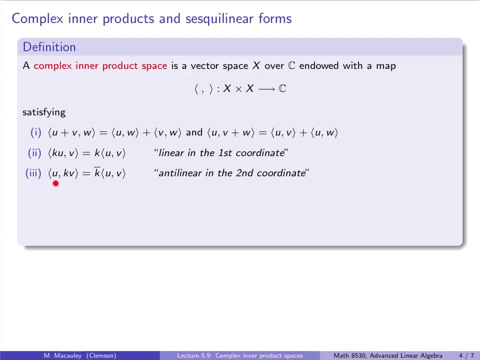 but you have to put a bar on front. In other words, the inner product of u and k with kv is k bar times the inner product of u and v. Sometimes this is said to be antilinear. in the second coordinate There's other terms as well. 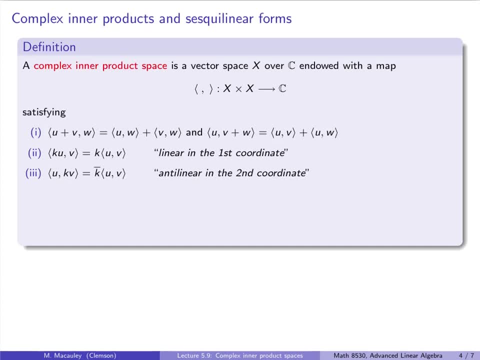 I forget what they are, but I like antilinear best. Four: we no longer have symmetry, but we have something close to it. When we swap the order of the entries, we have to take the complex conjugate, In other words the complex conjugate of v and u, the inner product of v. 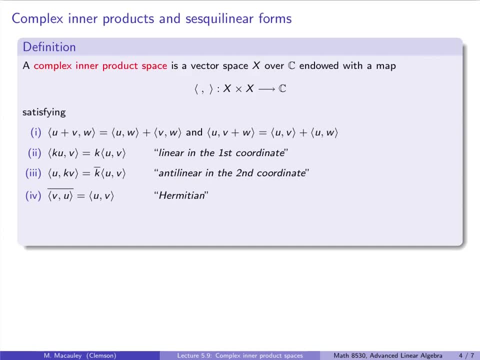 is the inner product of u and v plus the inner product of u and v, In other words, the complex conjugate of v and u. the inner product of v is the inner product of u and v, In other words, the complex conjugate of v and u, the inner product of v and v. 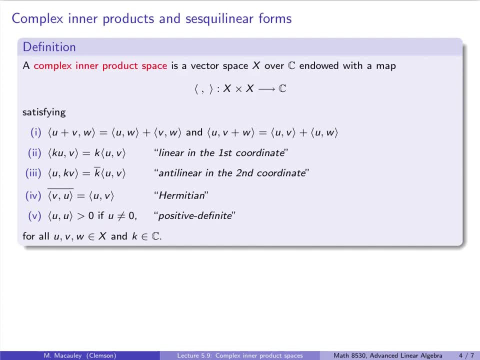 This is said to be Hermitian. And finally, like for real inner products, we need the condition of being positive, definite. So that is, the inner product of u with itself is positive if u is non-zero. So notice, I didn't explicitly say it's real. 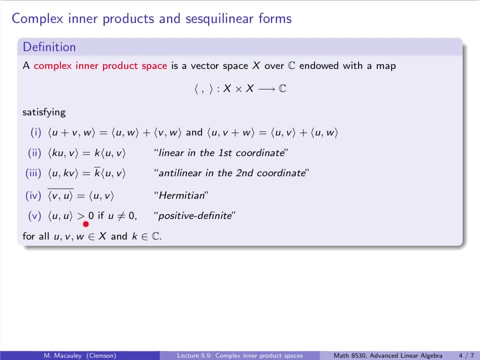 but the fact that I'm saying it's bigger than zero implies that it's positive. The complex numbers are not an ordered field. The complex numbers are not an ordered field. So these things hold for all. obviously: u, v and w, that are vectors and all scalars, k. 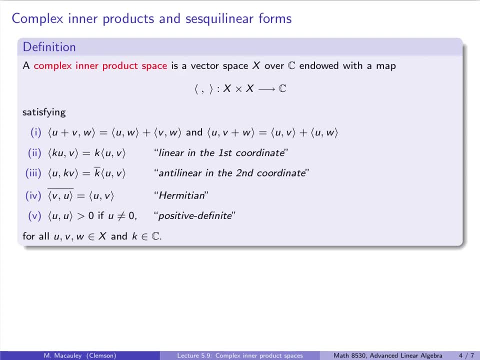 Now I do want to say: notice that this is not an alternate definition of a real inner product space. So if we restrict ourselves to vectors where the coefficients are real numbers, and scalars k where these are real numbers, and scalars k where these are real numbers, 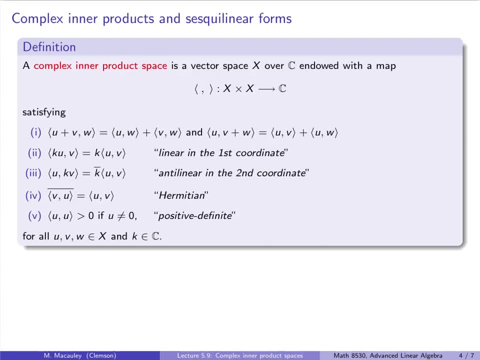 all of these, then our definition agrees with the definition of a real inner product space. In other words, if k is real v, So this is a bi linear. In other words, if k is real v, So it's a bi linear. 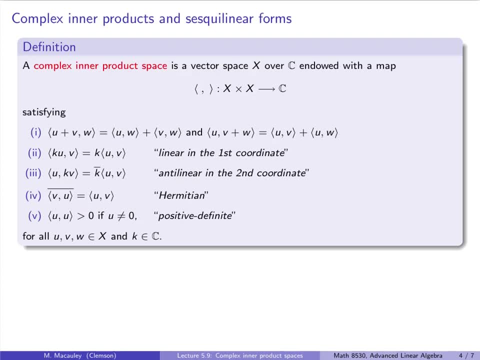 And it's also symmetric v, because the complex conjugate of any real number is itself. The first three conditions here are sometimes called sasquilinear, The first three conditions here are sometimes called sesquilinear, And in Latin that prefix sesqua, means one and a half. 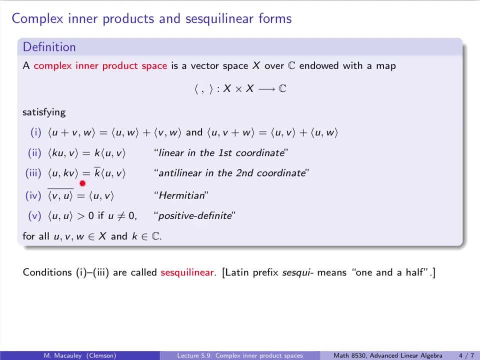 So I think it's a cute name. It's linear in the first coordinate and then it's sort of anti, or sometimes called semi-linear, in the second coordinate. So yeah, one and a half A map that is of this form, satisfying these first four conditions, is called a symmetric sesqualinear. 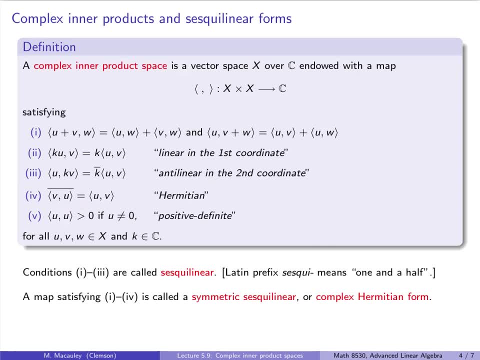 Sounds like a little bit of an oxymoron because this is not symmetric, but that's what it's called sometimes. Or a complex Hermitian form. So in other words, a complex inner product is a complex Hermitian form. that is also positive definite. 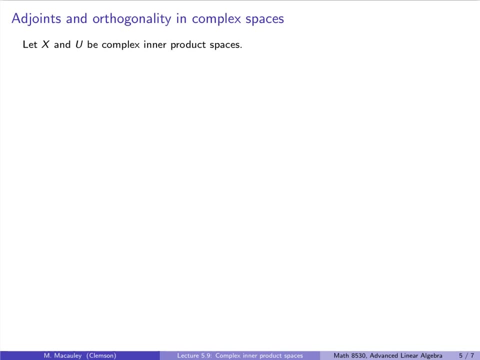 Now that we have defined a complex inner product structure, we naturally get notions such as adjoints and orthogonality, like we did in real vector spaces. Let's take a moment to understand what these mean, And it's important to realize that these are not alternative definitions. 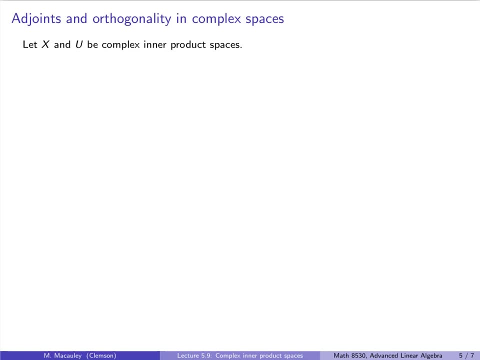 They are generalizations or extensions of our definitions for real inner product spaces. In other words, if we're in a complex inner product space but we're looking at vectors that are real, coefficients that are real, then our definition here should agree with what we had previously. 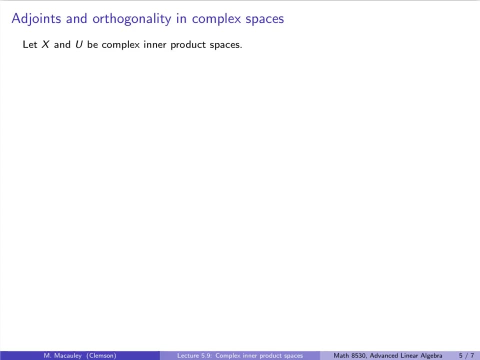 So let's let X and U be complex inner product spaces For any vector space. we have to have a complex inner product space For any vectors: X and Y, the norm of X plus Y squared. remember how that's defined. that's the inner product of X plus Y, with X plus Y. 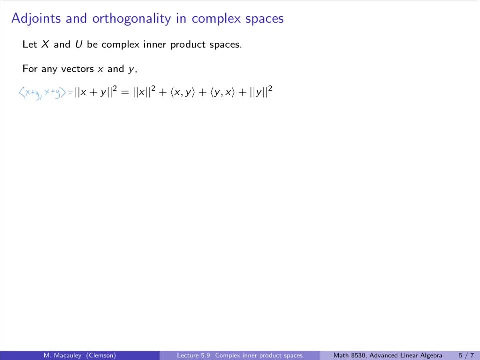 So we can use the additivity property to write that as the inner product of X with X, which is just the norm of X squared, plus the inner product of X with Y, plus the inner product of Y with X and the inner product of Y with Y. 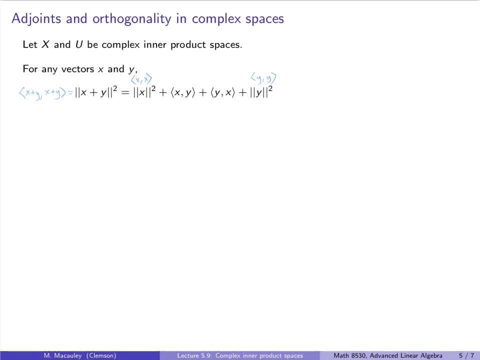 which is the norm of Y squared. Now, in the real case, this is symmetric, so we could combine this and we could write this as 2 times the inner product of X and Y. However, we don't have that when we're in a complex inner product space. 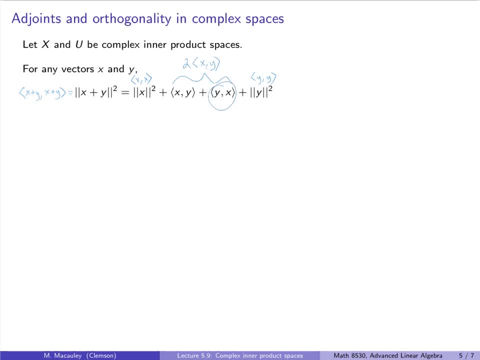 Remember that the inner product of Y with X is the conjugate, complex conjugate, of the inner product of X. So we can write this as 2 times the inner product of X with X squared, plus the inner product of X with Y. 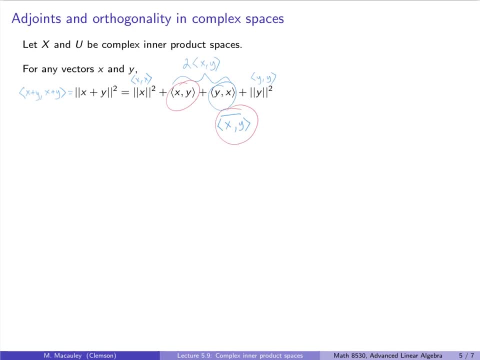 So now, instead, we have the sum of these two things and remember what that is in the complex plane. So if we have a vector z, which is a plus bi, and we add it to z bar, which is a minus bi, 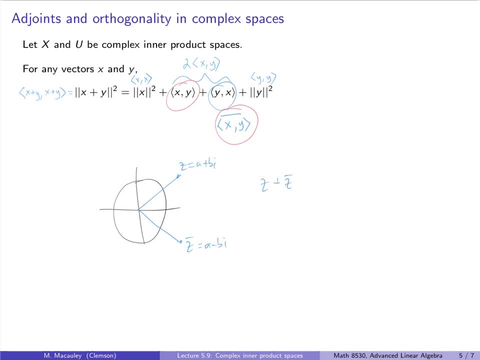 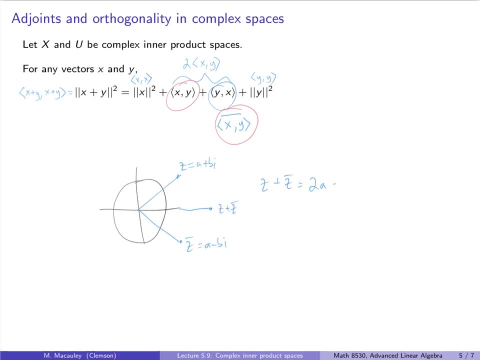 So this is z plus z bar, which is 2 times the real part of z. So, instead of this being 2 times the inner product of X with Y, it's 2 times the real part of the inner product of X with Y. 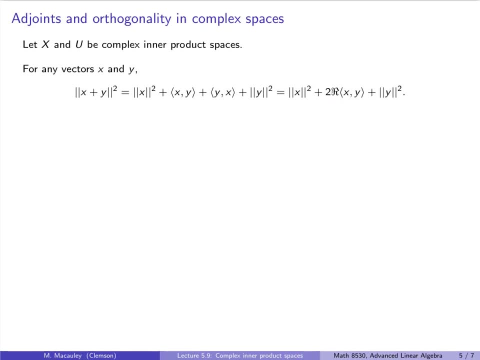 And we use this gothic R to denote the real part. Notice that if we're in a real vector space, or if the inner product of X with Y is real anyways, then this just reduces. then this just reduces to 2 times the inner product of X plus Y. 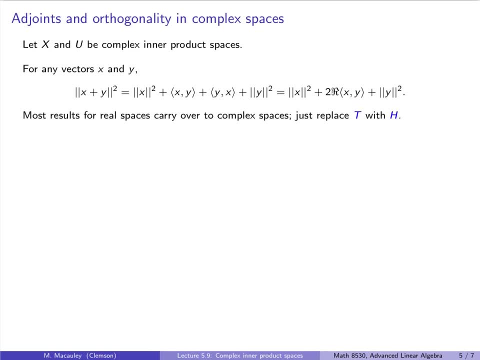 then this just reduces to 2 times the inner product of X plus Y. Most results for real vector spaces carry over to complex spaces and all we have to do is just replace T for transpose with H for Hermitian. and all we have to do is just replace T for transpose with H for Hermitian. 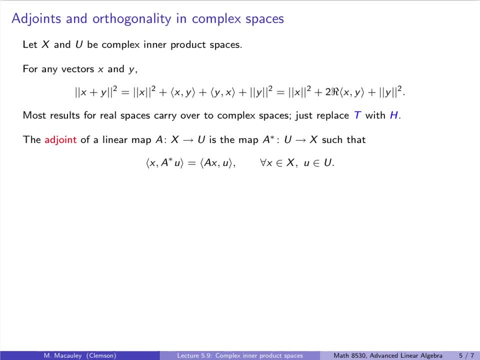 For example, the adjoint of a linear map A from X to U is the map A star from U to X, such that the inner product of X with A star U equals the inner product of AX with U, for all X and X and U and U. 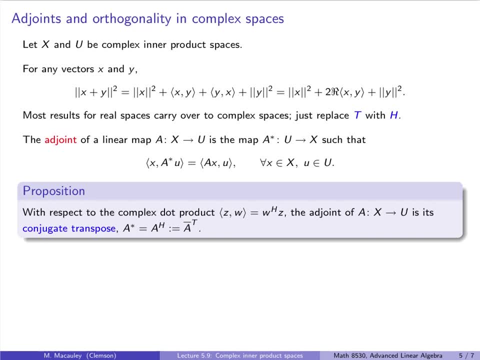 It should come as no surprise that, with respect to the complex dot product that we defined earlier, the adjoint of A is its conjugate transpose, That is, in matrix form. Now let's just write down why that's true. I should say that this definition I wrote up here. 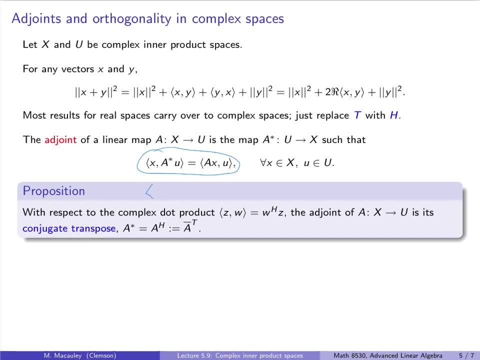 is obviously equivalent to just saying X comma A. U equals A star, X comma U. It doesn't really matter which one of these we use. basically we have to put the star. basically we have to put the star Anytime we move the a from the left to the right side. 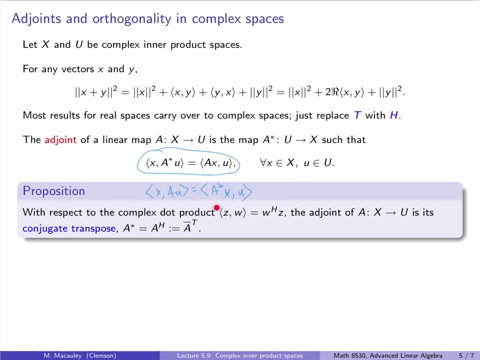 or vice versa, we have to put a star on it. So actually I think this version is slightly easier to verify this, though they're basically the same. Let's just write down x dot au. This is uha hx, And if this is equal to a star, x dot u. 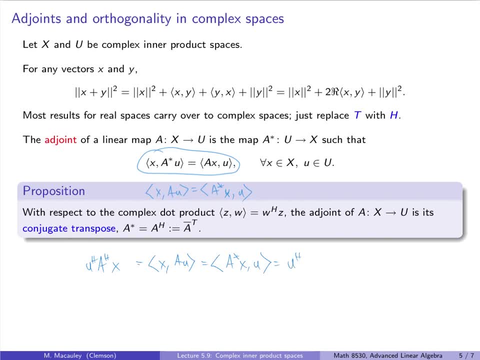 then this is, uh, a star x, And so for these two things to be equal- the left-hand side and the right-hand side- then it's obvious that ah has to be equal to a star. Now, that's if you use This definition here. 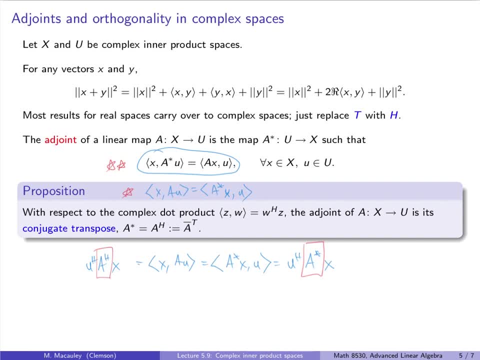 If you use this first one up here, then I think what you'll get is that a, You get basically the same thing. you get a star h. uhx equals uha x. So basically here you get that a equals a star h, and if you just apply h both sides- 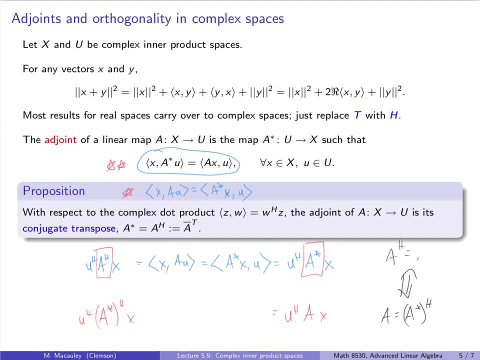 That's the same thing as saying a h equals a star, So take your pick as to which one of these you like best. The takeaway message is that in matrix form, the adjoint is the conjugate transpose And once again, this is not a different definition. 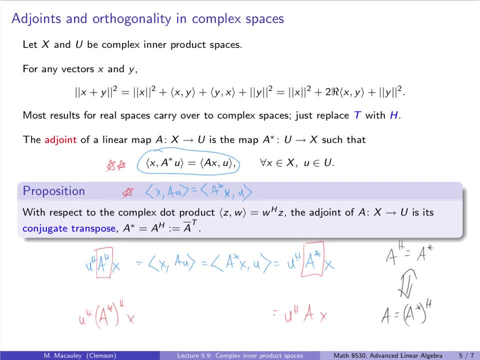 from a real vector space case. It's just a way to extend it. So if everything is real valued, then you get the transpose as before. One thing you may be wondering is what if we use a different inner product? so the example that I've done before is at least for real vector spaces where the inner product 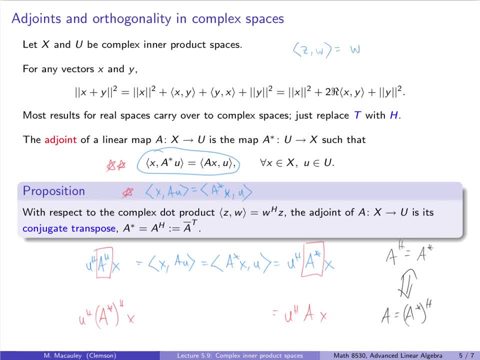 is defined as w and for real spaces I did w transpose, but let me do wh times, some matrix b, z, so we can certainly have a positive definite matrix in here to make things different. and so in this case the adjoint is not going to be the conjugate transpose, I think it'll be like a. 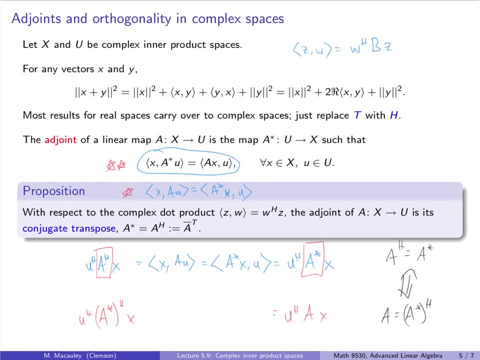 comp it'll be a conjugate of the con, of the conjugate transpose of a, but I think I will leave that as a homework exercise. Also, we will see later in this class that it doesn't matter which inner product structure we use. if we pick an orthonormal basis, then everything behaves. 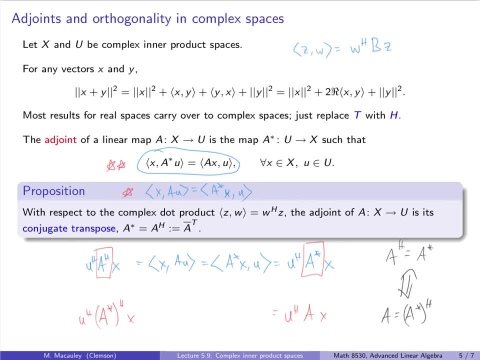 just like that, Just like a complex dot product. So in other words, given any inner product, we can treat it just like a complex dot product, and so we can treat the adjoint as the conjugate transpose. Let's move on to orthogonality. So the definition is basically the same as. 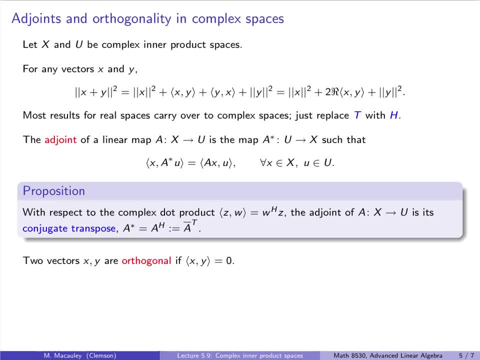 in the real case, Two vectors, x and y, are orthogonal if their inner product is zero. The vectors x- one up to x k- are orthonormal if they are pairwise orthogonal and have unit length. So in other words, if the inner product of x i and x j is the Kronecker delta. 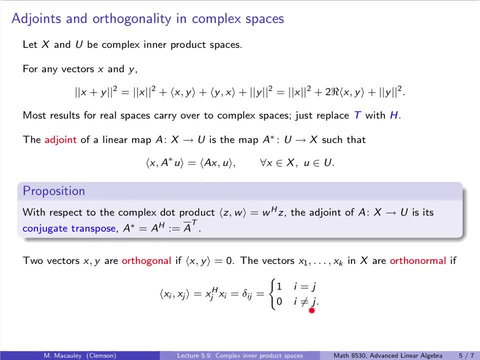 that is one if i and j are the same and zero if they are different. So the only difference here is: if the vectors x and y have complex enterports, then the inner product is also entries. you just got to be careful that when you take the inner product you take the conjugate. 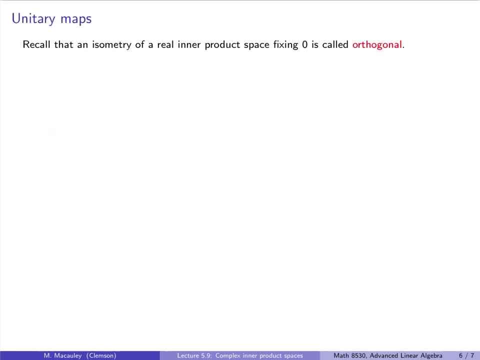 transpose. Recall that an isometry of a real inner product space that fixes the zero vector is called orthogonal. An isometry of a complex inner product space fixing zero is called unitary. I really don't know why they use different terms for this, especially because we have a notion of 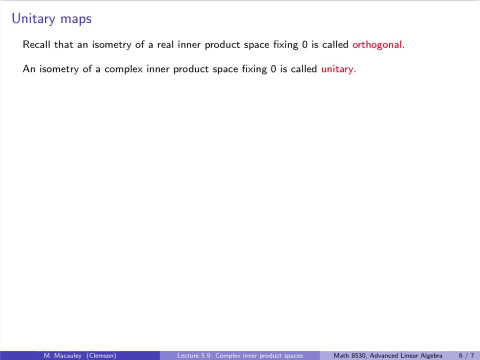 orthogonality of vectors in an inner product space. but it is what it is. Since we call a real-valued matrix A orthogonal if A transpose A is the identity. we will call a complex-valued matrix unitary if AHA is the identity. Basically, the term orthogonal means that the adjoint of a 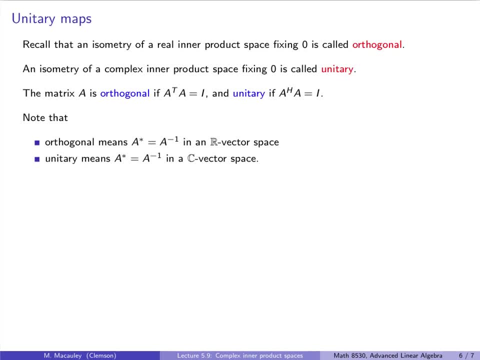 vector space is unitary, and unitary means the same thing, but in a C vector space. Now, this definition of orthogonality, this is not a relation that we really ever care about holding in a complex vector space. So you could definitely write down a matrix where this thing 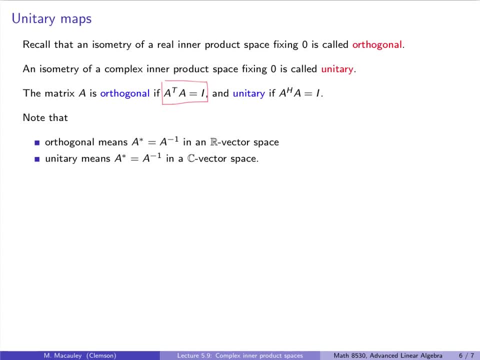 holds in a complex vector space and that will not have the property that this holds. but we don't really care about that, So we're just going to assume that any time we're talking about a matrix we're talking about orthogonal matrices, that they are real-valued. Here's a quick proposition. 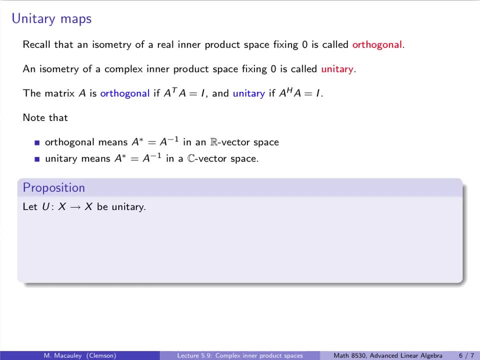 which we basically established for real vector spaces and orthogonal maps. Go back and watch that lecture, and the proofs carry on almost exactly the same here, just you have a slightly different meaning as to what A star is, So let U be a unitary map from a vector space to itself. 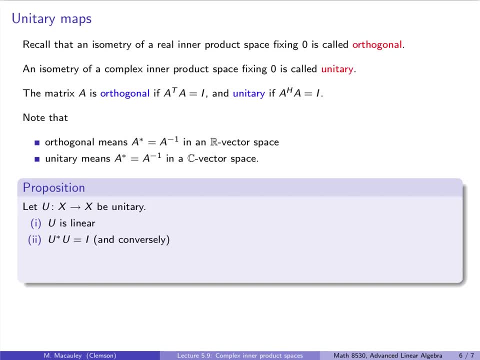 Then U is linear, U star, U is the identity and conversely, U is invertible and its inverse is an isometry. Finally, we have that the determinant of U is a complex number with norm 1.. In other words, 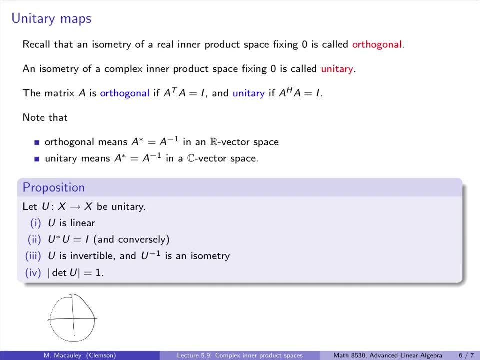 it lies on the unit circle, So it's of the form e to the i theta. for some theta Now, what we had previously for orthogonal maps is that the determinant of A was plus or minus 1. So that's a special case of being on the unit circle and also being 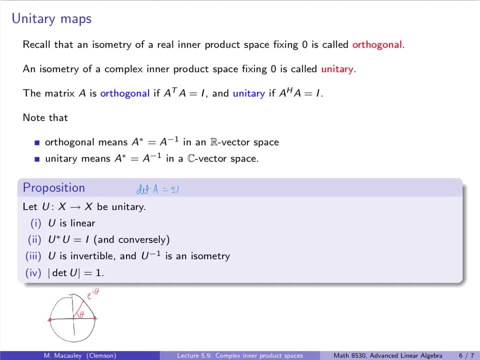 real. So the reason why this one is true Is because U star U equals the identity. so the determinant of U star U equals the determinant of U star times. the determinant of U? u equals the determinant of the identity, which is 1.. 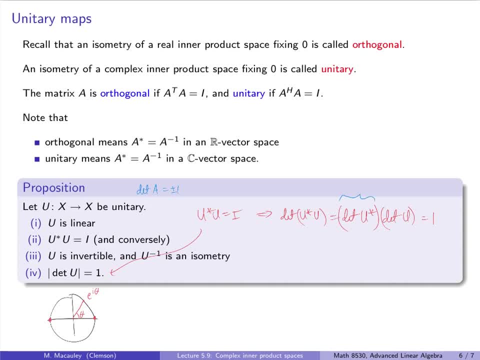 And I guess one thing that I haven't proven but I will leave as a simple exercise is to show that the determinant of u star is the complex conjugate of the determinant of u. So you need these things together. So determinant of u is a complex number, e to the i theta, such that it times its conjugate. 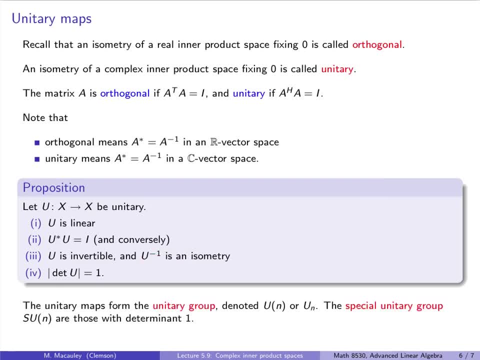 is equal to 1.. Finally, the unitary maps form the unitary group often denoted u of n or u sub n, where n is the dimension And the special unitary group s u of n are those with determinant exactly 1.. 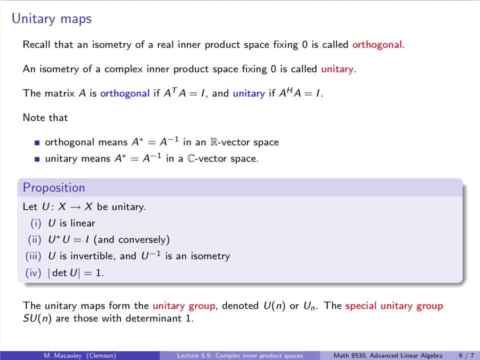 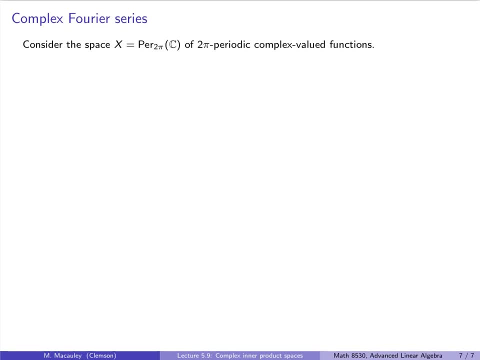 So you think of those as complex rotations and the other as complex isometries. I'll finish this lecture with an application to Fourier series. Previously in this class, in several different lectures, I've introduced the idea of Fourier series, And this is a way to write a periodic function as an infinite sum of sine and cosine waves. 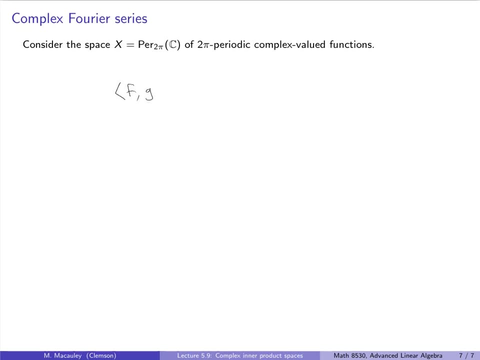 And there I defined an inner product between functions f and g as 1 over pi times negative pi to pi. f of x, g of x, dx. Now everything was real valued. so I didn't put a bar on top of g, g of x, because I didn't need to. 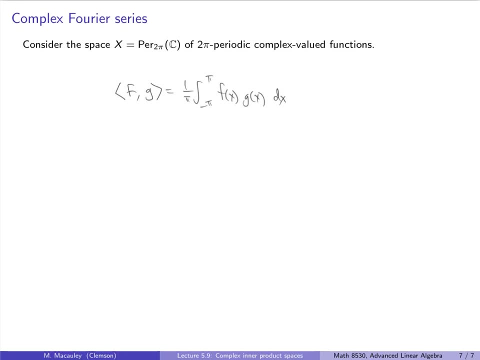 And with respect to this inner product, if you recall the cosine functions, cosine of x, cosine of 2x, et cetera, and the sine function, sine of x, sine of 2x, et cetera, this infinite, 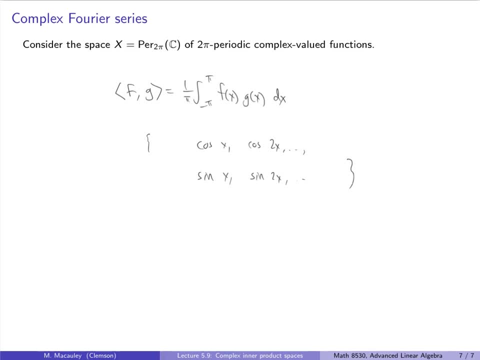 set was not only a basis but an orthonormal basis, That is, I left out a constant function, Actually unfortunately 1. It does not have unit length, So 1 over root 2 has unit length. So this is an orthonormal basis, which meant that every periodic function can be represented. 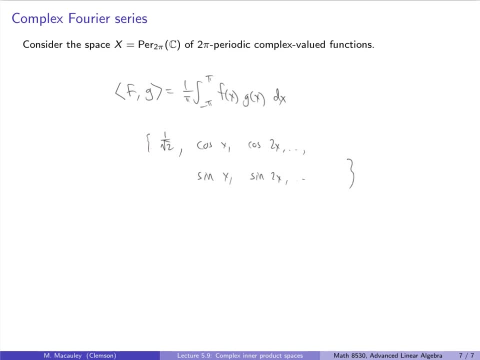 uniquely as a sum of sine and cosine waves and possibly a constant. So there's this weird constant out here. I mean it has to be there, but the fact that it has to be normalized by root 2 is kind of an artifact of the fact that we are using sines and cosines instead of the much more 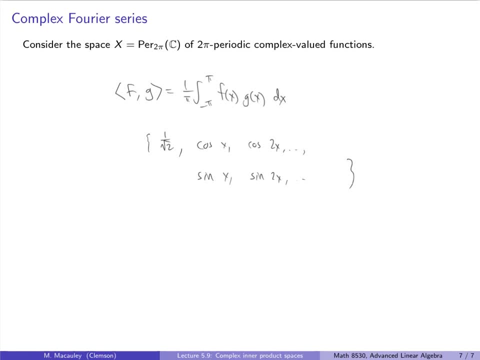 natural, And so it's a very complex exponential. So recall that cosine of nx is e to the i? nx plus e to the minus i nx over 2, and sine of nx equals e to the i? nx minus e to the minus i nx over 2i. 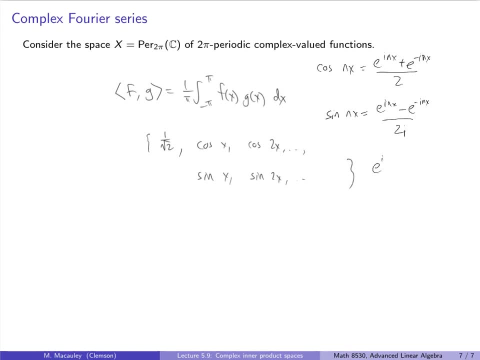 And similarly you can go the other direction by saying e to the i nx is cosine of nx, plus i sine of x, OK, sine of nx. So you could actually go between these two spaces by just turning cosines and sines into exponentials, or vice versa. However, for the inner product to work, 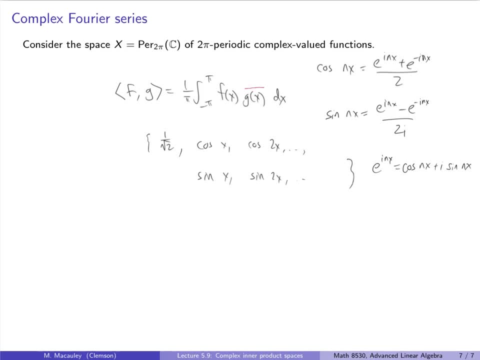 you're going to need to put a bar right there. And also, if you do that, if you put a bar here and define it like this, your complex exponentials are not going to actually have unit length. If you want to make them have unit length, you have to divide by 2 pi instead of pi. 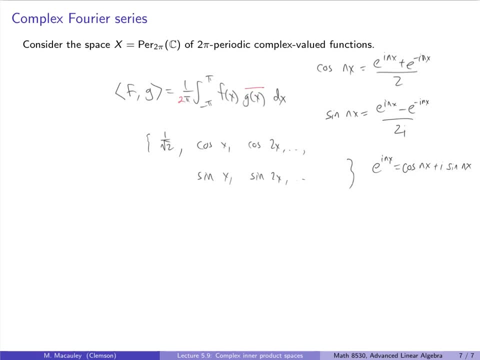 So let me go through and say that a little bit differently, Because if you haven't seen Fourier series before, if you haven't watched my old videos, then what I just talked about probably isn't going to make too much sense. So, starting from scratch, we can define an inner product on the space of 2 pi. periodic functions. 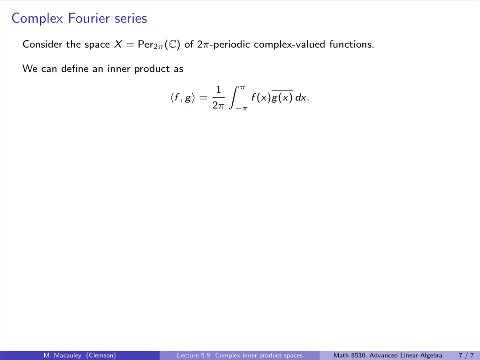 As follows: the inner product of f and g is 1 over 2 pi times the integral from negative pi to pi. basically one complete cycle of f of x times g of x, bar dx. With respect to this inner product, the following infinite set of complex exponentials, e to the i and x, where 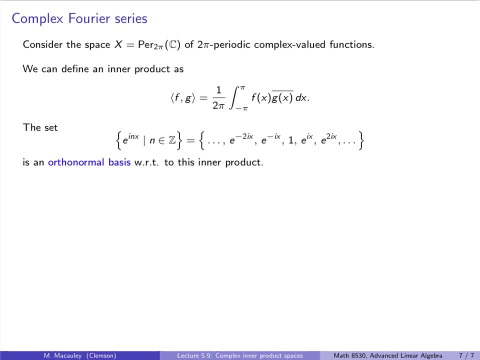 n are integers, positive and negative, and 0, which gives you 1,. this is an orthonormal basis with respect to this inner product. Therefore, we can write each f of x in this space uniquely, as this doubly infinite sum, from negative infinity to infinity, of cn i to the n? e to the i n x.